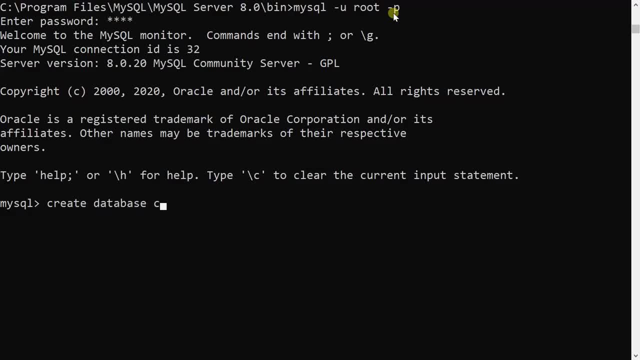 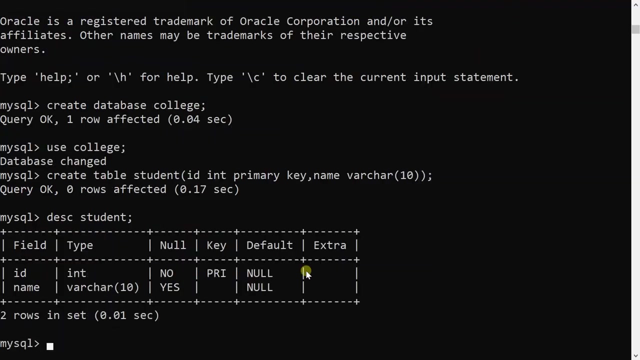 database college. I will use the database and under this college database I will create one table, student- with two attributes only Because I want to show how to grant permission, how to revoke permission. So here my table is created. I can see the structure of the table here. Ok, So now I 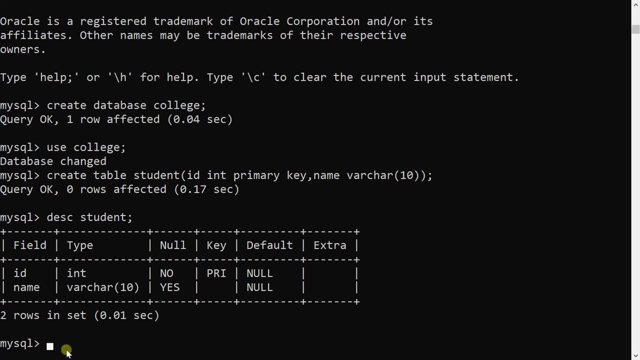 will create user. So how many users to be created? Number of users can be created. Right, I will create user using command CREATE USER And CREATE USER is DDL statement Data Definition Language. Because we are using CREATE WORD, CREATE USER is used to create user, So I will. 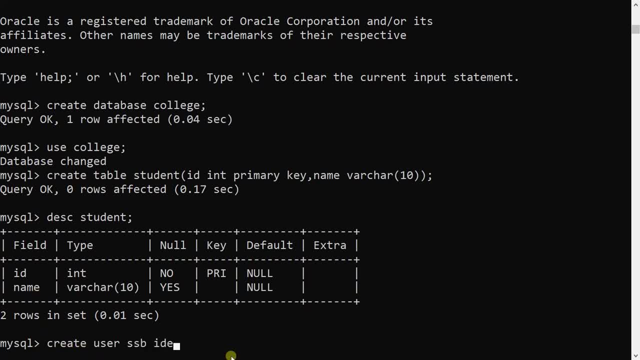 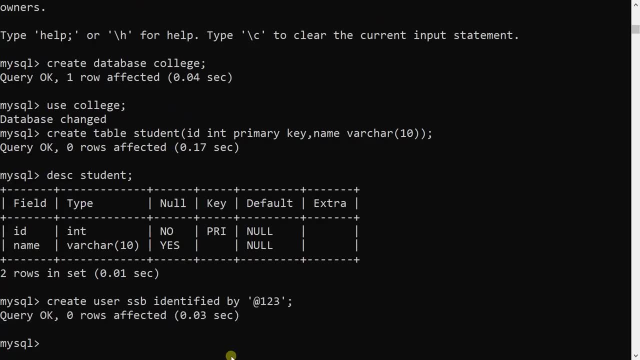 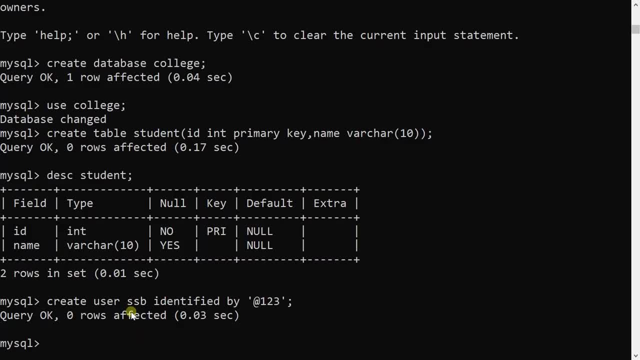 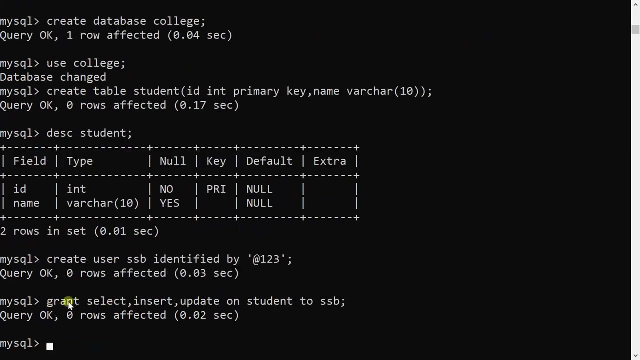 If I want to grant permission to user, like which operation can be performed by that user. it can be done by using GRANT command, GRANT SELECT, Then Insert and update. i am showing you three commands or three operations are granted on which table, student table, to which user ssb. so what does it mean? what this command means? it 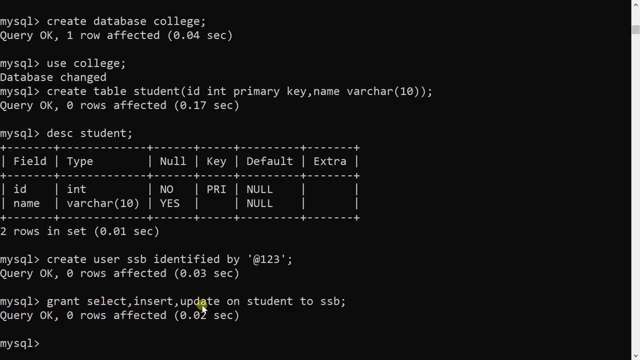 means three operations: select, insert and update are granted on table name: student on table, student to ssb user. so ssb can perform select operation, insert operation and update operation on student table. and student table is under college database. so now here i will show you how ssb will work on. 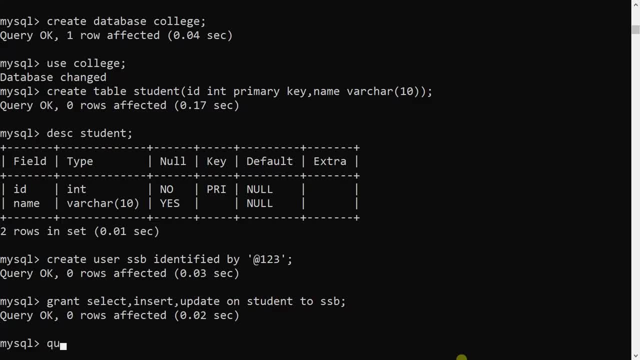 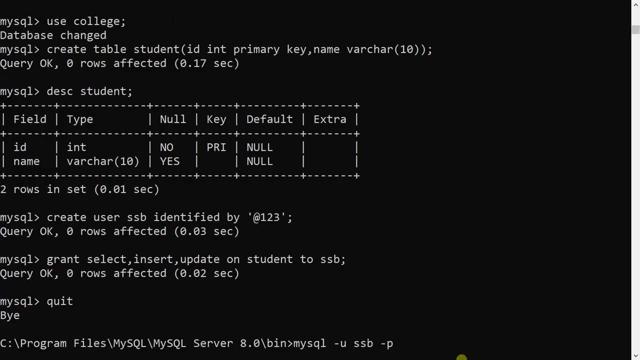 these three operations. so what is to be done? i will quit from this root here. instead of root, i will type ssb, because one user has been created by root here. here it will operate on the ssb user. so now i will show you how ssb will work on these three operations. 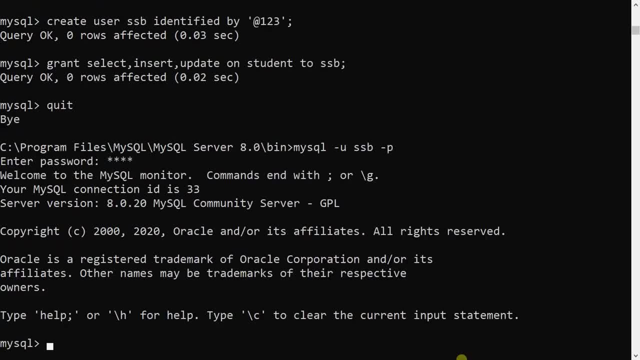 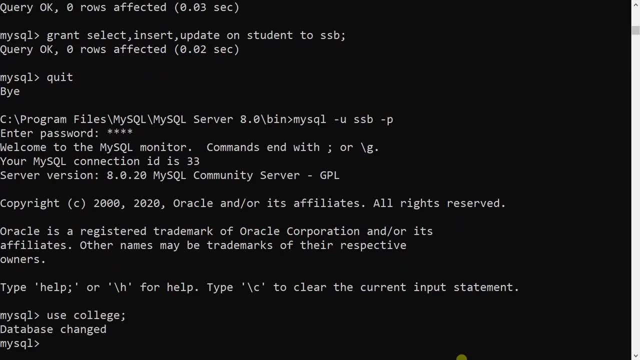 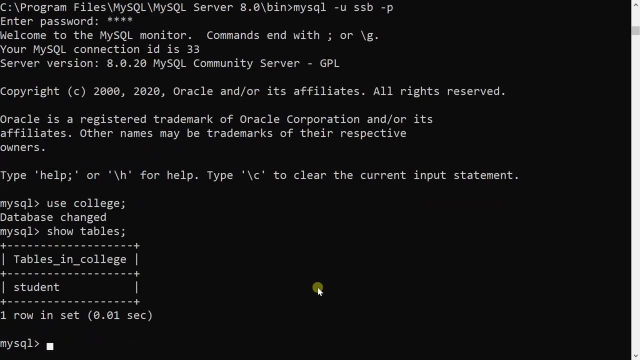 ask for password, so i will enter the password. so now i am in ssb user, i will use that college database and here i will execute command: show tables. so here, friends, you can see only one table has been created under college database. so ssb user can see student table. so three operations. 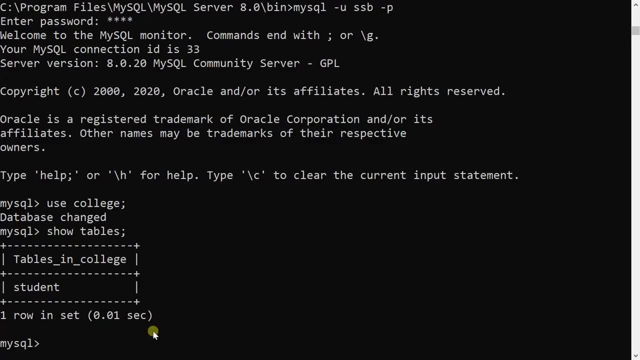 can be performed by ssb user. so the first one is insert. insert into student. what are the attributes? id and name values. one, abc. the second, pqr. third, id is acting as a primary key, so we need to insert unique record key. so we need to insert unique record key. 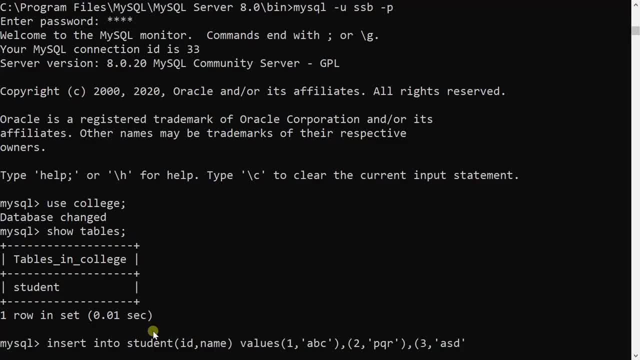 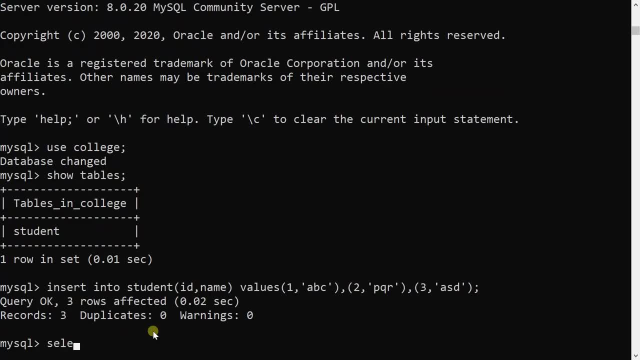 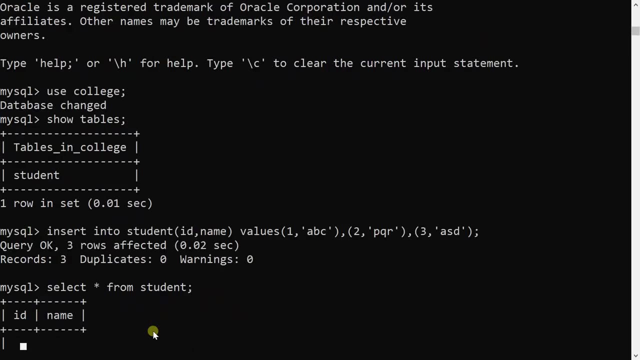 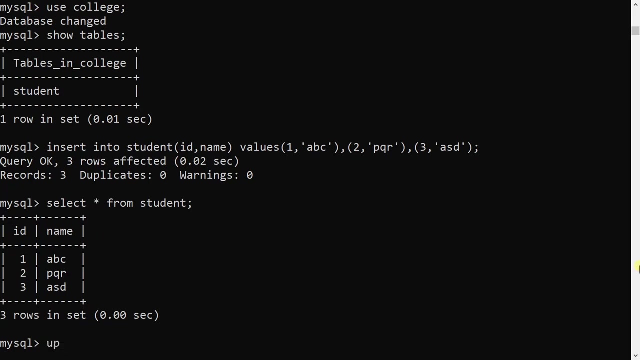 for id. so i have inserted three records. insert permission was granted. even select permission is granted so i can execute select star from student. so here you can see select operation is also done successfully. update operation is also granted to ssb user so i can execute update command. 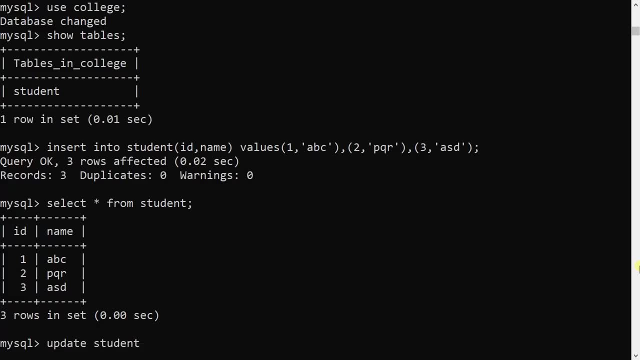 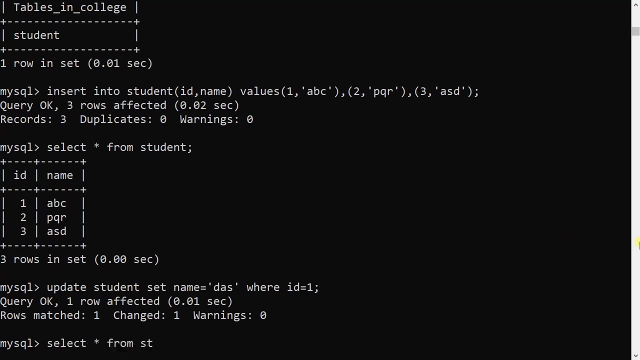 also update what is to be updated. table student said: if i want to update name, name is equal to as, or i will say ds where id is equal to 1. so here you can see query. ok, i will execute select star from student. so, friends, here you can see the changes. what was the query? update student. 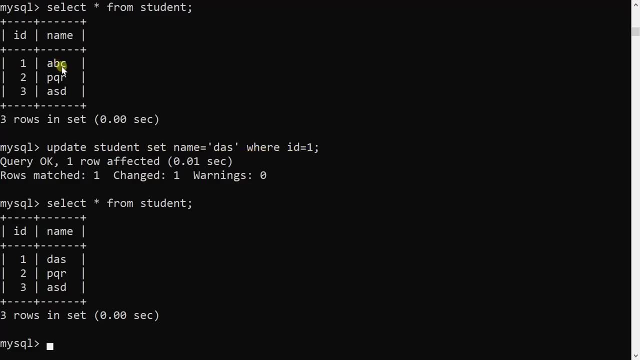 set name is equal to, thus where id is equal to 1, so from abc it is updated to das. so three permission were granted: select, insert and update. now i will execute delete statement. delete from student where id is equal to 1. so this command will not be. 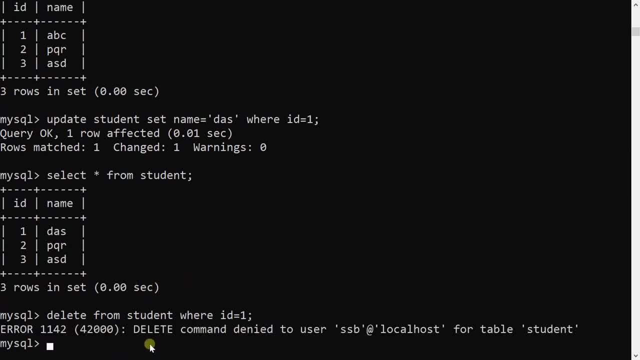 executed. delete from student where id is equal to 1, so this command will not be executed. executed by SSB, This error will come. delete command denied to user SSB for table student right because when SSB user is created, only three Operations were granted to SSB. That's what delete command could not be executed. 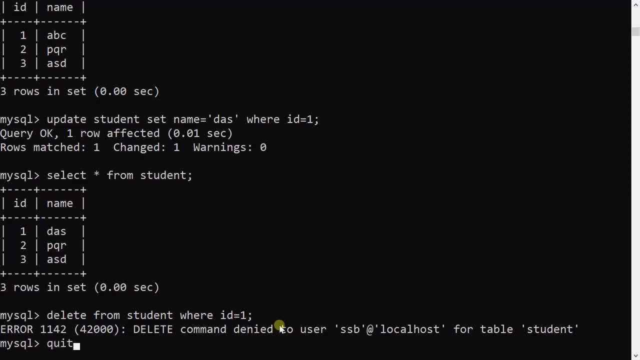 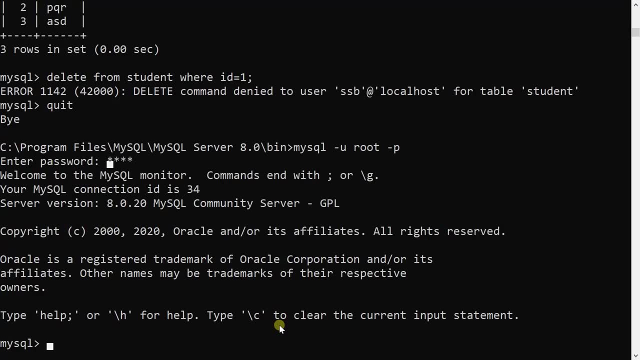 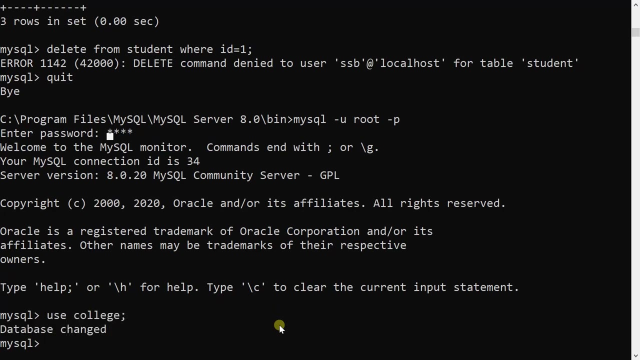 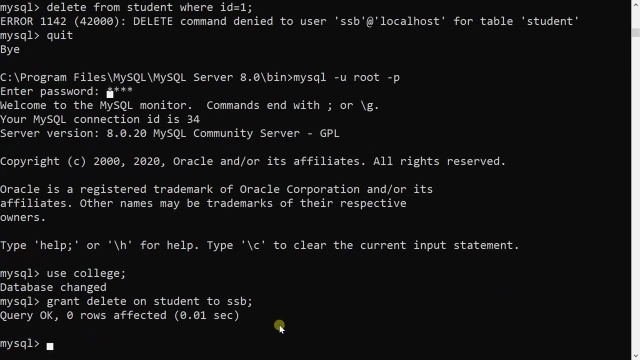 right. so if I say quit and I will go to root command again, I will use college database and I will grant delete permission to SSB, grant delete on Student to SSB. So query: ok. So now again we will check whether delete operation is performed or not. 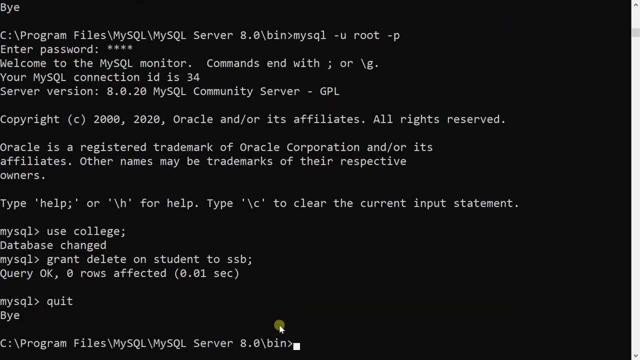 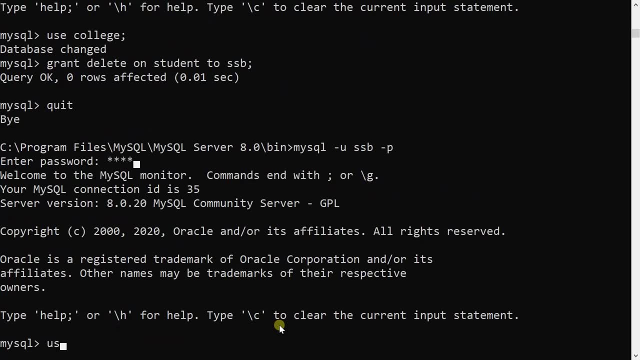 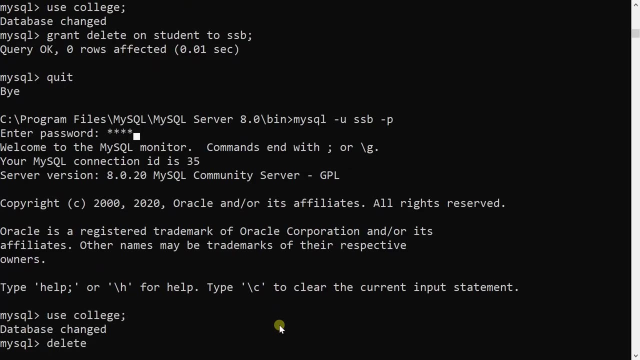 So again, I will have to quit from root. I will go to SSB. It will ask password. I will enter a password, I will use college database and I will perform delete operation- Delete from Student. before that, I will execute select so that we can see the changes. 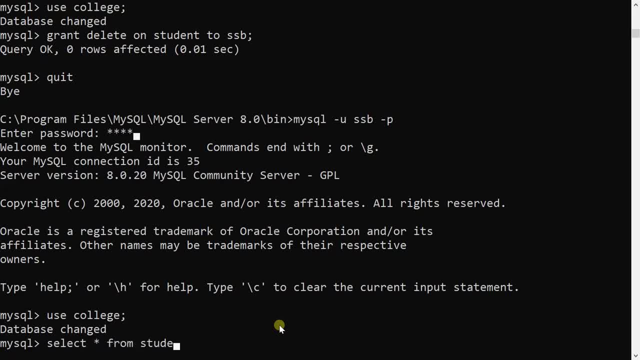 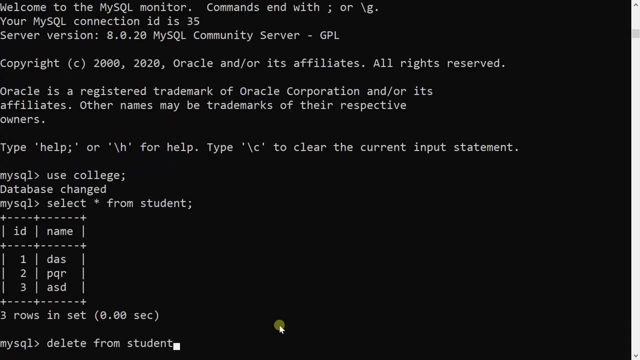 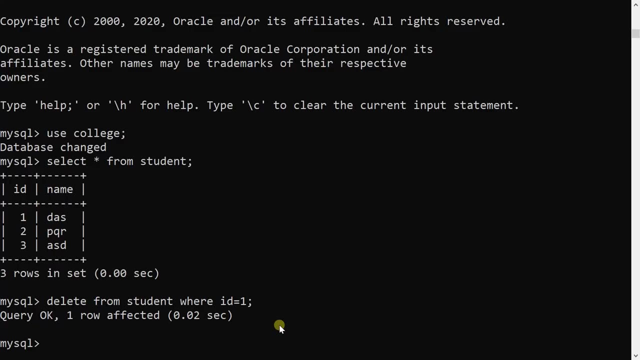 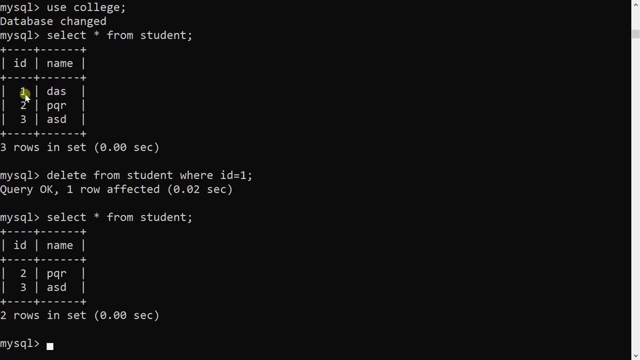 select star from student. Okay, so I will like delete a particular record. delete from student. delete from student where id is equal to 1. so query: okay, right. if i execute select star from student, you can see record number 1, where id is equal to 1, is deleted, right, so? 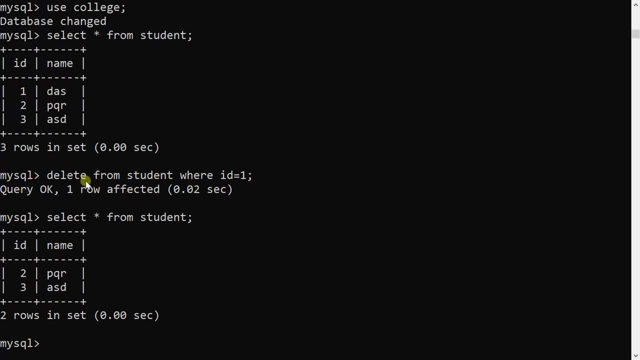 to ssb delete operation or delete permission has been given by root. that's what ssb can delete record from the student table. so all four operations can be performed by ssb. if root wants to revoke all the permissions from ssb, how it will be done, that i will show you. 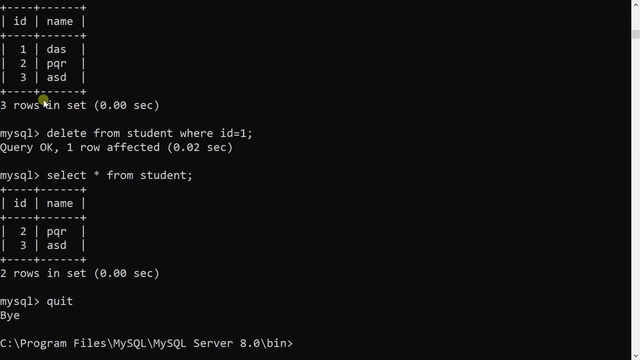 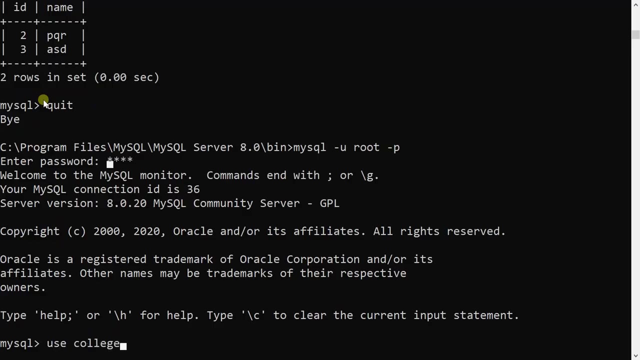 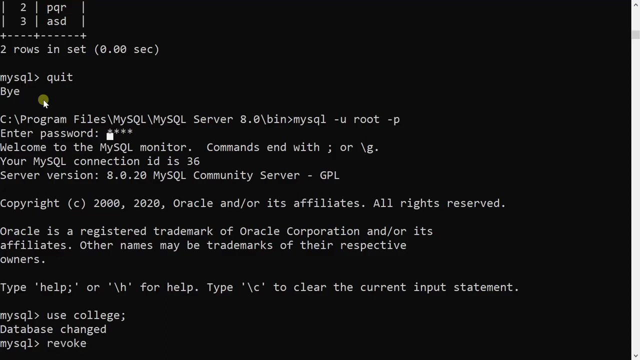 again we will have to quit from ssb because ssb is one user. granting and revoking permissions will be given by root only. again, i will enter into root, i will enter password, i will use password database and then i will revoke permissions from ssb. revoke select. i will show you two. 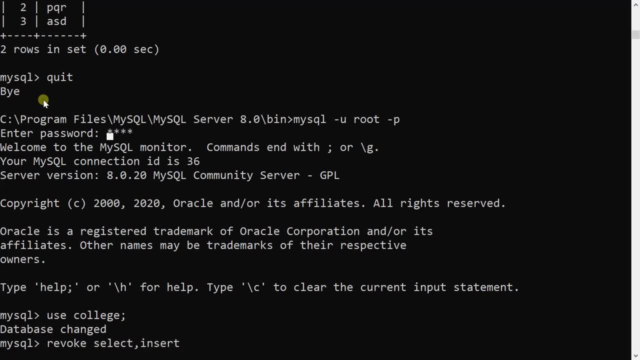 permissions, two operations that are revoked from ssb: revoke, select, insert. or i will show you: insert and delete from on which table. remember to specify on which table they've given its permissions for each console, so you must, delicious, to specify on which table the permissions are given. revoke, insert, delete. 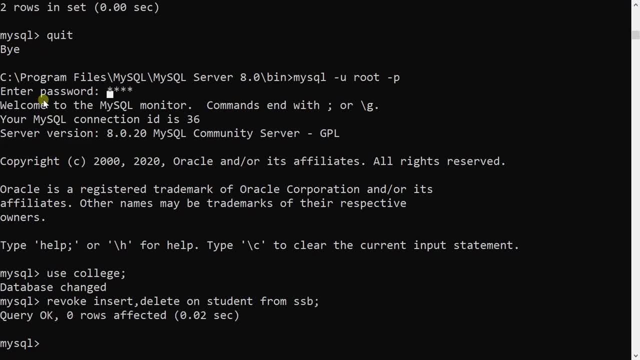 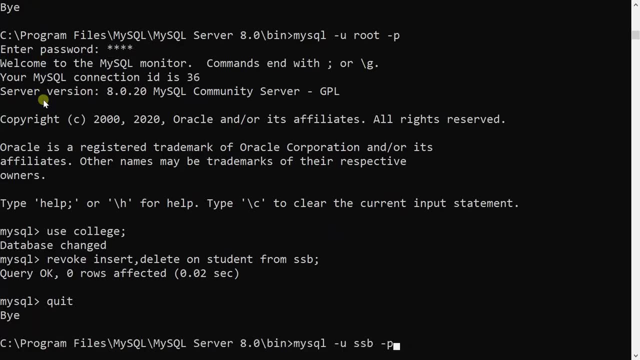 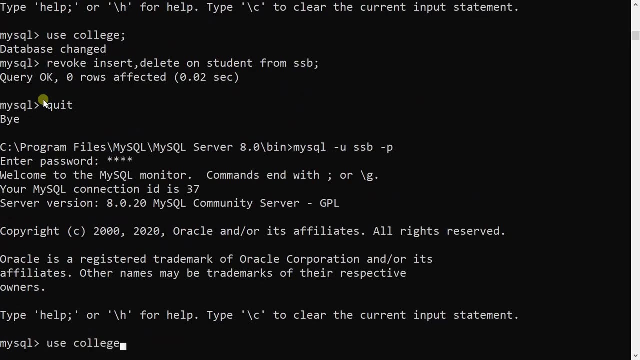 on student from ssb. so my query is: ok, whether the changes are done or not, that can be seen from ssb user only. so again, i will have to quit from root. i will enter into ssb. it will ask for password. i will enter password. i will use database enter. my intention is to make 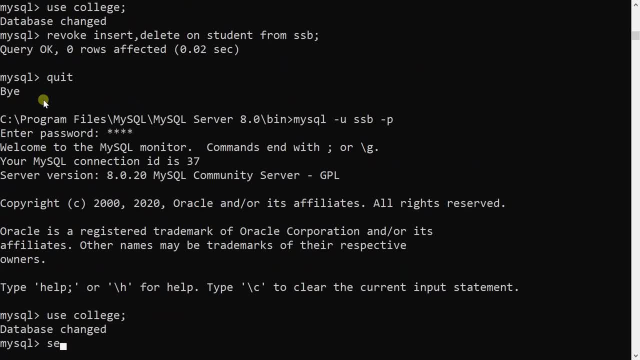 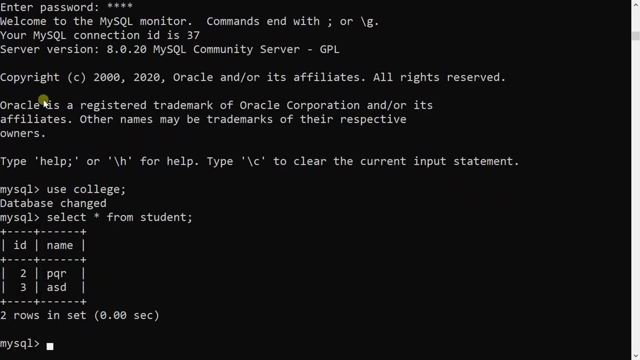 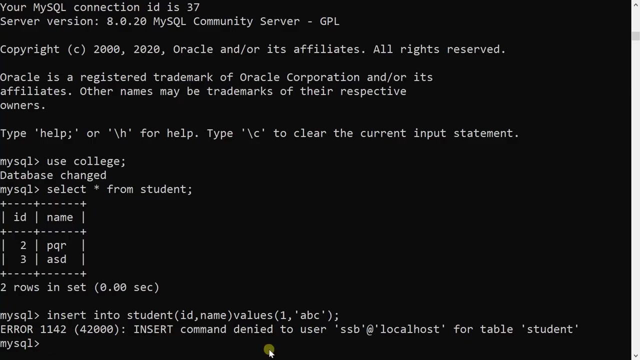 And here I will execute select statement: Select star from student. This statement will be executed because this permission is given. Two operations are removed from SSB: Insert and delete. If I insert record into student table, Insert into student ID, comma, name, values, 1 comma ABC, then inserted, because insert operation is revoked from SSB Right. Likewise, delete is also revoked. 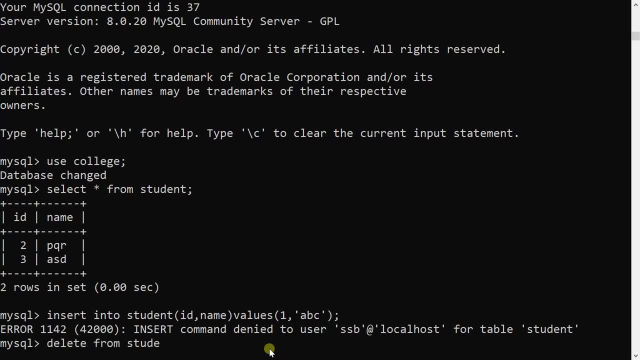 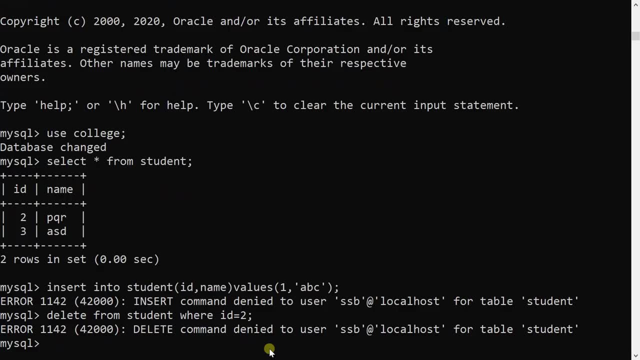 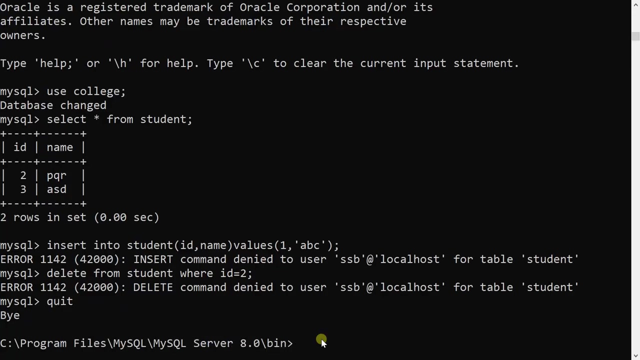 So if I execute delete from student Where ID is equal to 2.. Error Delete command denied to user Right. So two operations are revoked from SSB Right. So these are the two commands which I have shown you. If I quit from SSB, I will go to root.